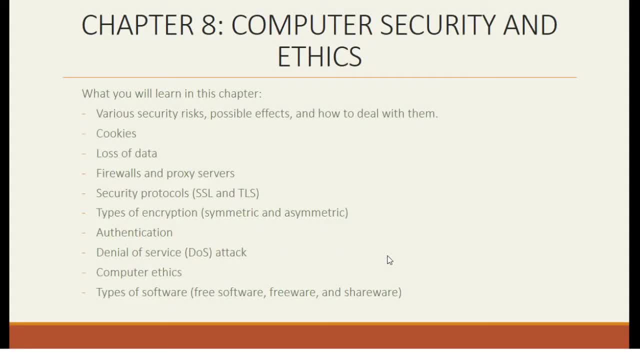 Welcome back to the IGCSE computer science code 0478 guide. This chapter we will be discussing about computer security and ethics. This chapter is quite lengthy, but not as long as chapter 5.. Before we start, the concepts you will learn in this chapter include the various security risks, possible effects. 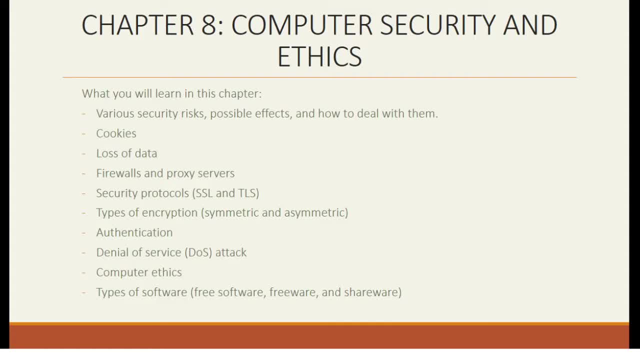 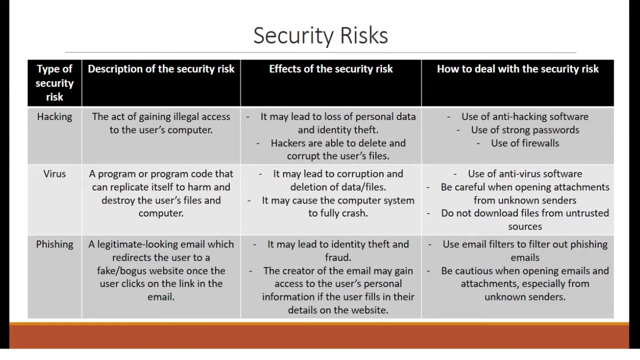 and how to deal with them: cookies, loss of data, firewalls and proxy servers, security protocols- namely SSL and TLS, types of encryption- which is symmetric and asymmetric- authentication, DOS attack, computer ethics and the types of software. Let's start with the security risks. In this chapter, you will be 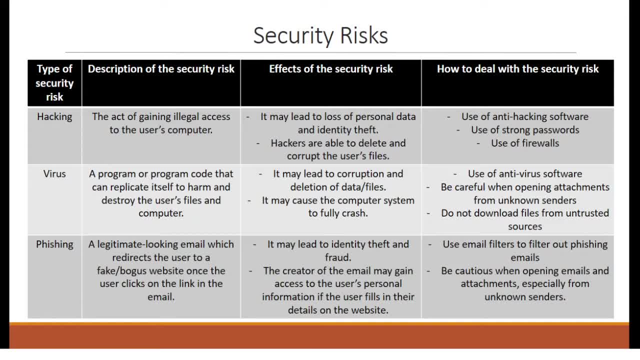 learning about six main security risks. First, hacking: It is the act of gaining illegal access to the user's computer. Its effects: It may lead to loss of personal data and identity theft. Hackers are able to delete and corrupt the user's files. And how to deal with them. 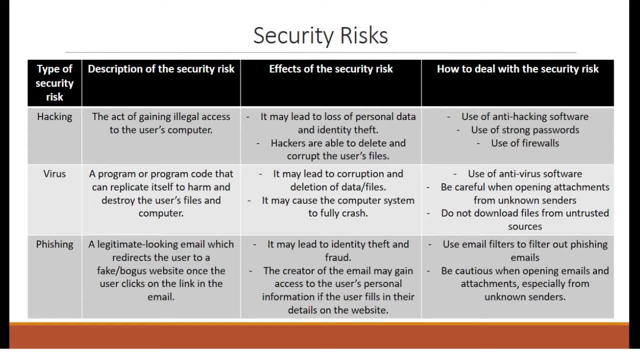 Use of anti-hacking software, use of strong passwords and use of firewalls. Virus: A program or program code that can replicate itself to harm and destroy the user's files and computer. It may lead to corruption and deletion of data or files. 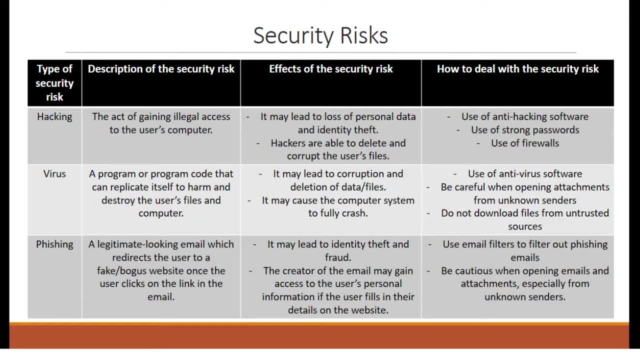 It may also cause the computer system to fully crash. To deal with them, use of anti-virus software. be careful when opening attachments from unknown senders and do not download files from untrusted sources. Phishing: A legitimate looking email which redirects the user to a fake or 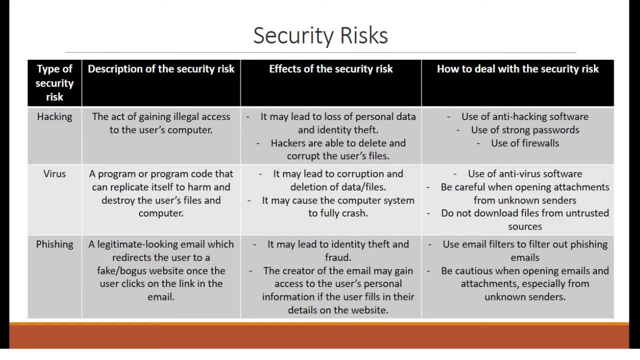 bogus website. once the user clicks on the link in the email, It may lead to identity theft and fraud. The creator of the email may gain access to the user's personal information if the user fills in their details on the website. To deal with them use email phishing. 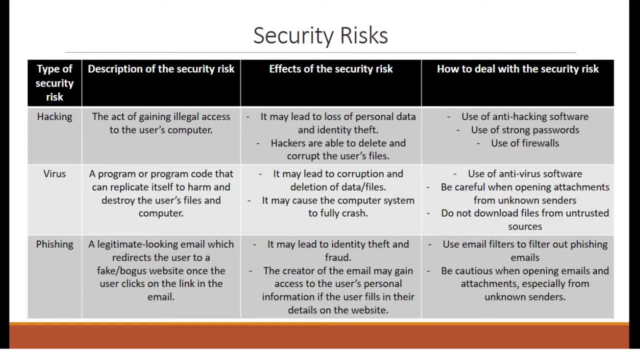 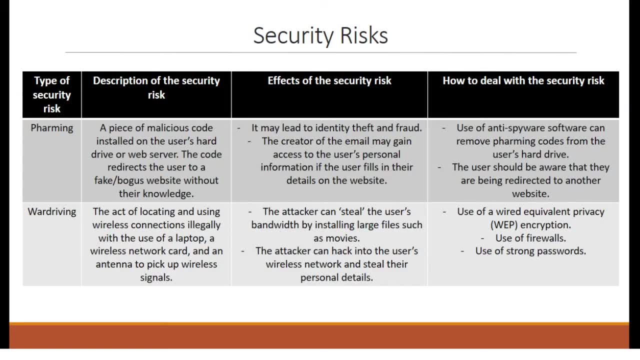 Use phishing to filter out phishing emails and be cautious when opening emails and attachments, especially from unknown senders. Farming A piece of malicious code installed on the user's hard drive or web server. The code redirects the user to a fake or bogus website without their knowledge. It may lead 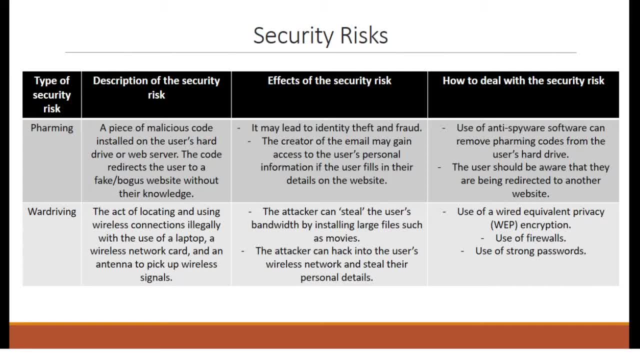 to identity theft and fraud. The creator of the email may gain access to the user's personal information if the user clicks on the link in the email To deal with them. use of anti-virus software. be careful when opening attachments from unknown senders To deal with them. use of: 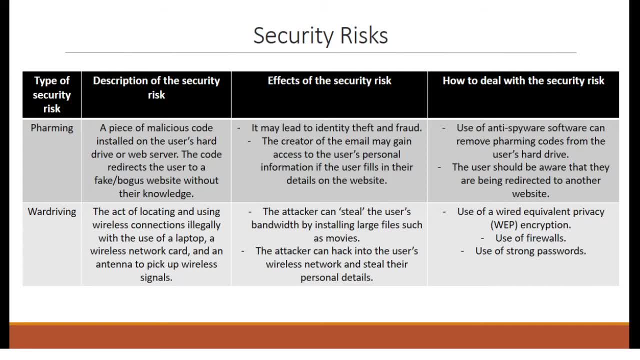 personal information if the user fills in their details on the website to deal with them. use of anti-spyware software can remove farming codes from the user's hard drive and the user should be aware that they are being redirected to another website. who are driving? it is the act of locating. 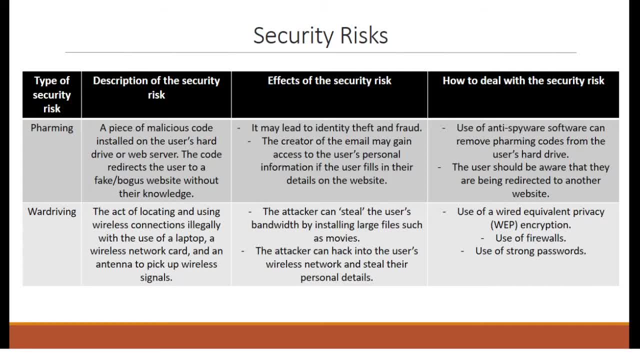 and using wireless connections illegally. with the use of a laptop, a wireless network card and an antenna to pick up wireless signals, the attacker can steal the user's bandwidth. by installing large files such as movies, the attacker can hack into the user's wireless network and steal their personal details. to deal with them, use of a wired equivalent privacy or wep encryption. 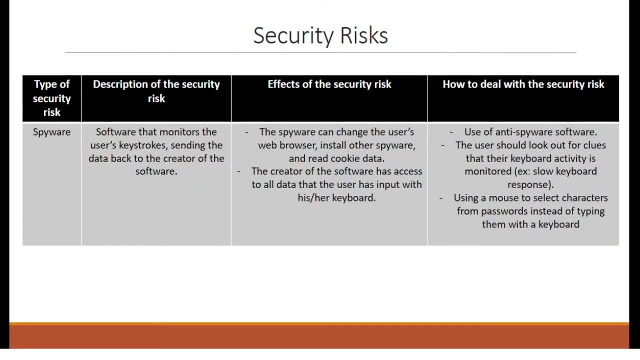 use of firewalls and use of strong passwords. spyware: it is software that monitors the user's keystroke and the user's memory. the attacker can also hack into the user's wireless network, sending the data back to the creator of the software. Spyware can change the 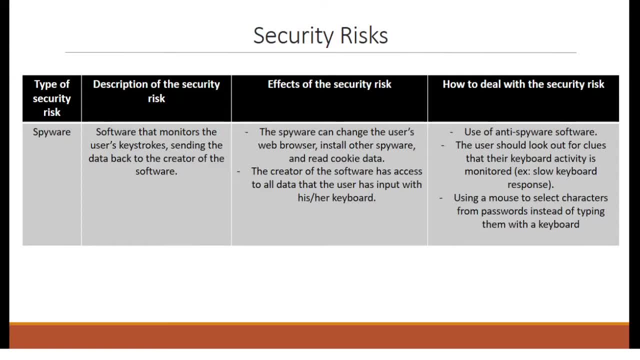 user's web browser, install other spyware and read cookie data. The creator of the software has access to all data that the user has input with his or her keyboard. How to deal with them? Use of anti-spyware software The user should look out for. 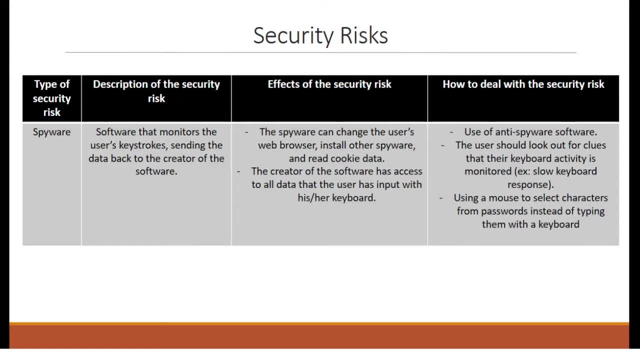 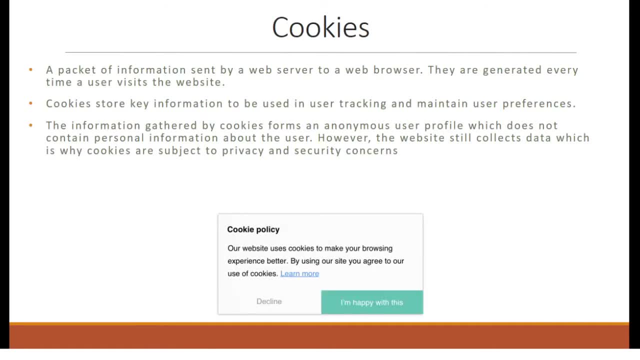 clues that there are keyboard activities being monitored and using a mouse to select characters from passwords instead of typing them with the keyboard. Cookies: It is a packet of information sent by a web server to a web browser. They are generated every time a user visits the website. Cookies store key. 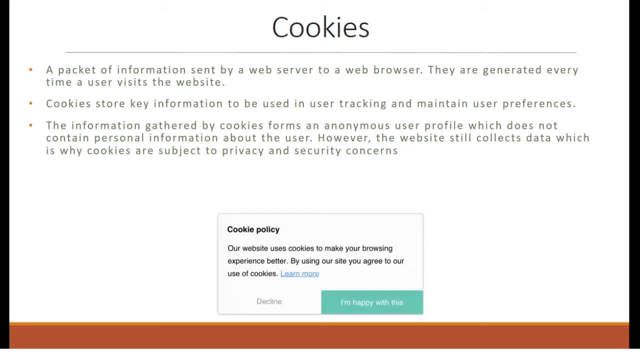 information to be used in user tracking and maintaining user preferences. The information is stored in a web browser. The information is stored in a web browser. The information gathered by cookies forms an anonymous user profile, which does not contain personal information about the user. However, the website still collects. 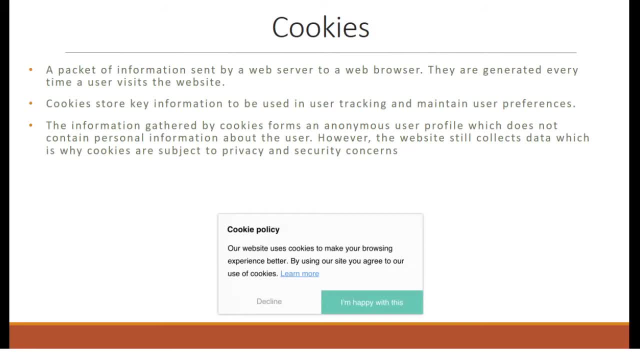 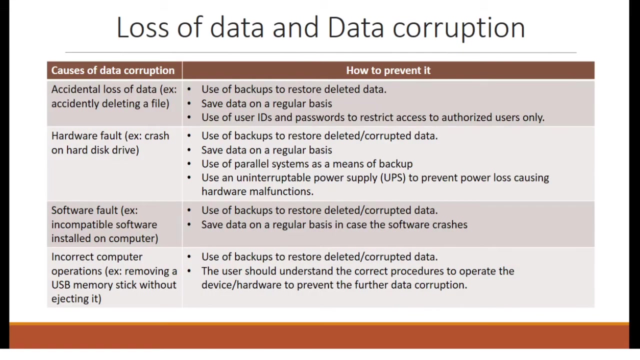 data, which is why cookies are subject to privacy and security concerns. An example of the usage of cookies is when a user purchases a video game from a website. The cookies remembers the user's buying habits and displays messages such as customers who bought cookies. A user who bought a game has also bought game XXX. 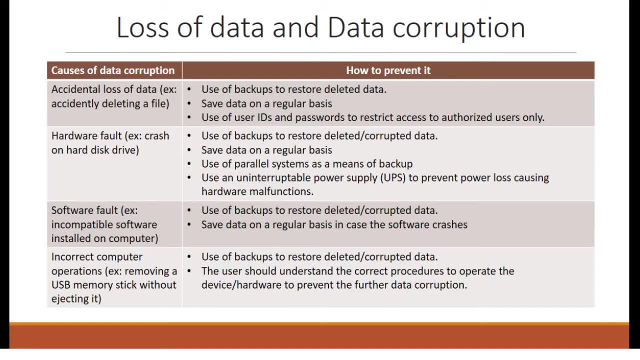 Moving on to the causes of data corruption and how you can prevent them: Accidental loss of data, such as accidentally deleting a file To prevent it. use of backups to restore deleted data, save data on a regular basis and the use of user IDs and passwords. 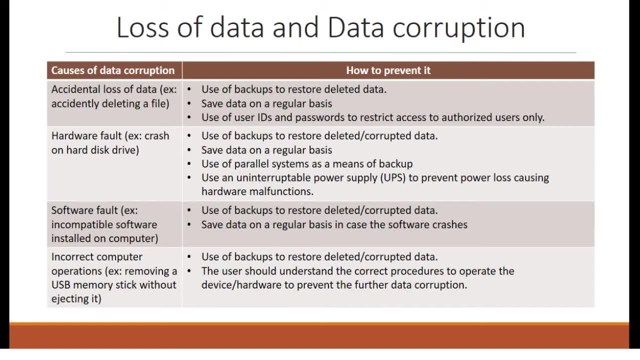 to restrict access to authorized users only. Hardware fault, Such as a crash on the hard disk drive. Use of backups to restore deleted or corrupted data. save data on a regular basis. use of parallel systems as a means of backup and use an uninterruptible power supply or UPS to prevent power loss causing hardware malfunctions. 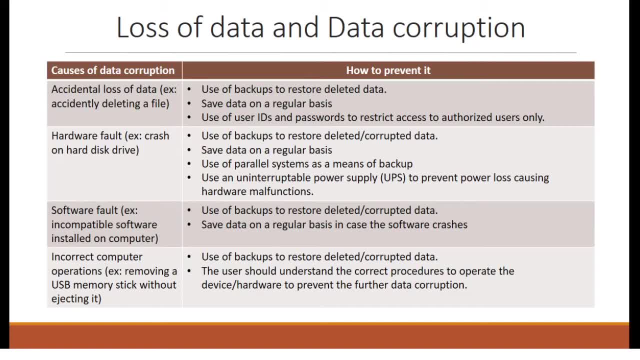 Software fault Incompatible software installed on a computer. Use of backups to restore deleted, deleted or corrupted data and save data on a regular basis in case the software crashes. incorrect computer operations, such as removing a usb memory stick without ejecting it. use of backups to restore deleted or corrupted data, and the user should understand the correct. 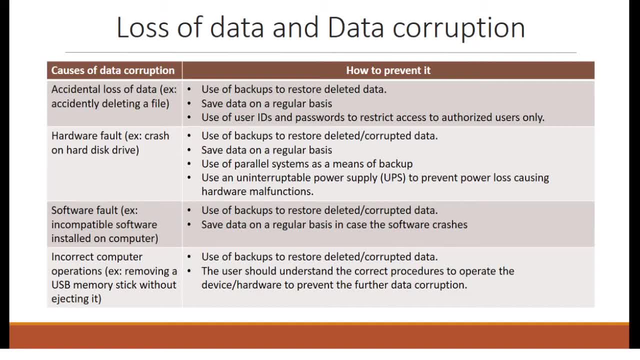 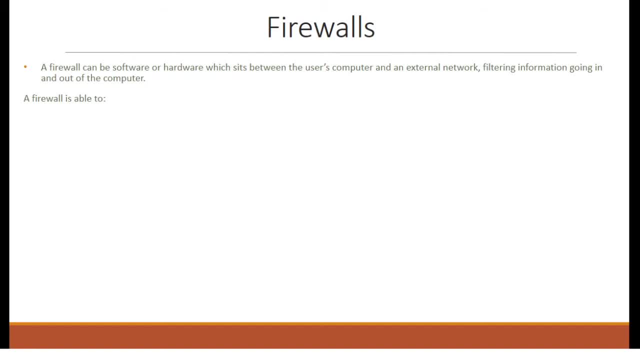 procedures to operate the device or hardware to prevent further data corruption. firewall: a firewall can be a software or hardware which sits between the user's computer and an external network, such as the internet, filtering information going in and out of the computer. a firewall is able to examine traffic between the user's computer and an external. 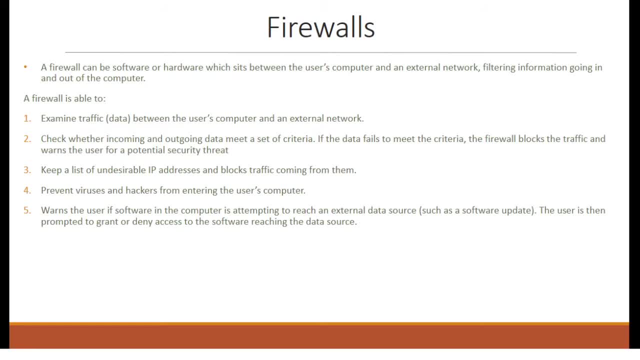 network. check whether incoming and outgoing data meets a certain meets a set of criteria. if the data fails to meet the criteria, the firewall blocks the traffic and warns the user for potential security threat. keep a list of undesirable ip addresses and blocks traffic coming from them. prevent viruses and hackers from entering the user's computer. 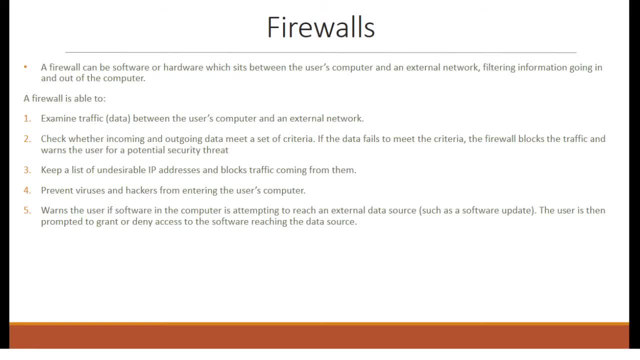 and warns the user if software in the computer is attempting to reach an external data source. the user is then prompted to grant or deny access to the software reaching the data source. however, a firewall cannot prevent users from choosing to bypass the firewall, leaving their computer vulnerable. prevent employee misconduct and carelessness, which 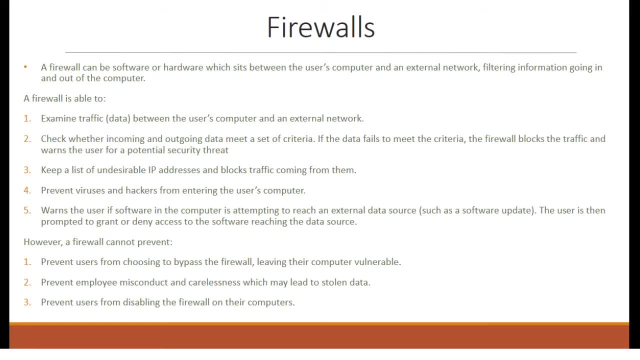 may lead to stolen data, and it cannot prevent users from disabling the firewalls on their computers. also, take note that a firewall can also exist as a hardware interface sitting on the computer's and a server-based network. for example, if you have an internet connection, this is referred to as a gateway. 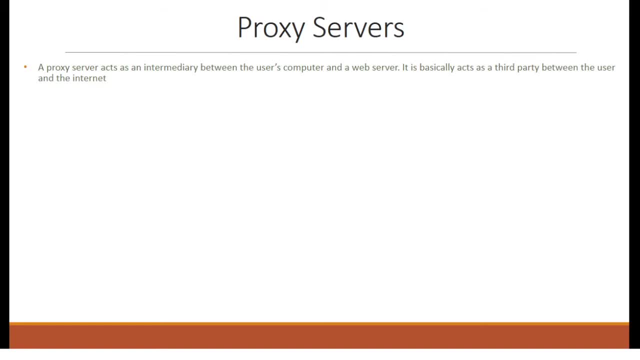 proxy servers. a proxy server acts as an intermediary between the user's computer and a web server. it is basically a third party between the user and the internet. the functions of a proxy server include filtering traffic going in and out of the computer, acting as a firewall and an internal network connection between the user's computer and the internet. 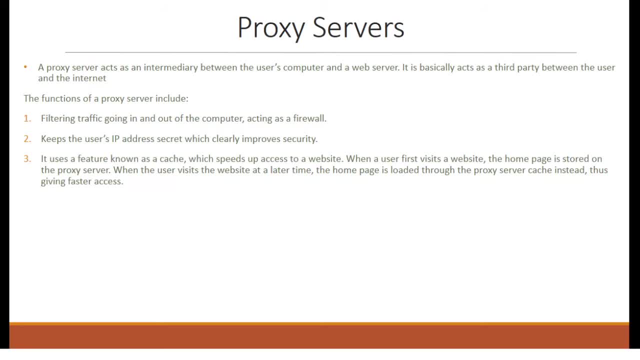 keeping the user's ip address secret, which clearly improves security, and it also uses a feature known as sash, which speeds up access to website. when a user first visits a website, the home page is stored on the proxy server. when a user visits the website at a later time, the home 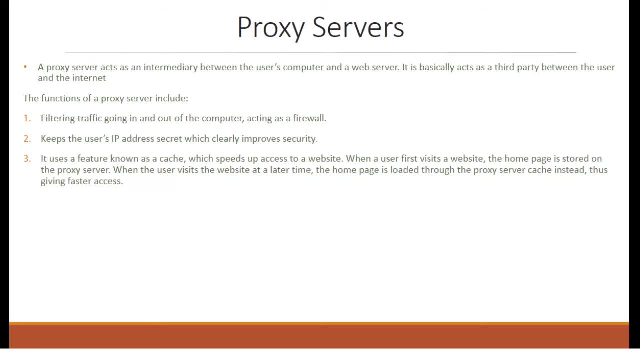 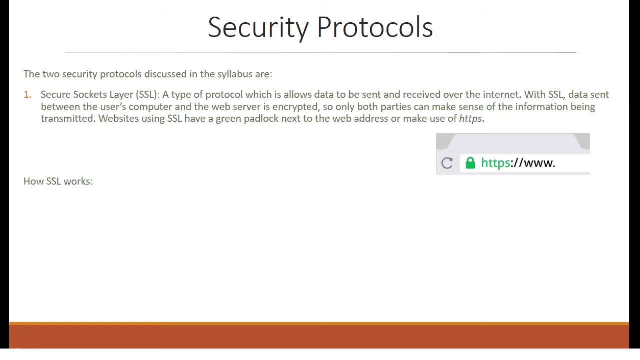 page is loaded to the proxy server cache instead, thus giving faster access. from the diagram below, we can see that the proxy server somewhat acts like a middleman between alice and bob. security protocols for the igcsc syllabus. we will be discussing about two security protocols. 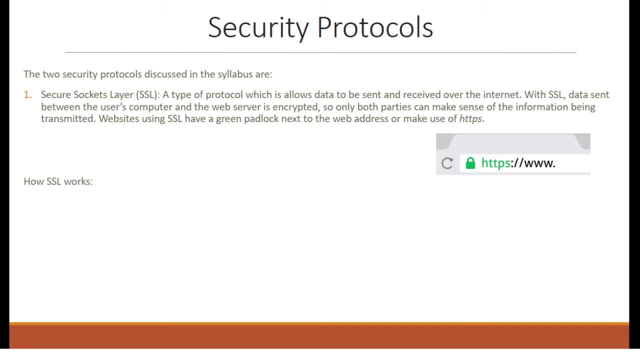 first, secure sockets layer or ssl. it is a type of protocol which allows data to be sent and received over the internet. with ssl, data sent between the user's computer and the web server is in the middle of the internet, and the data is then sent to the computer, and the web server is in the middle of the internet. 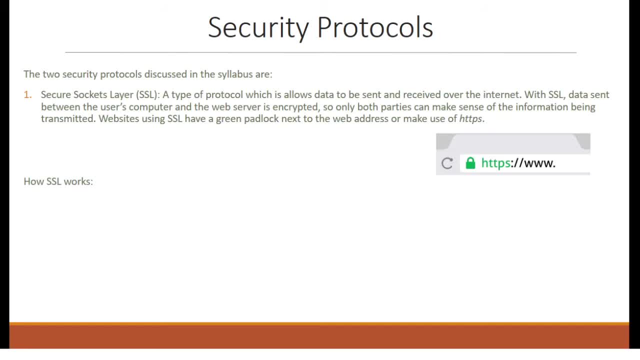 encrypted so only both parties can make sense of the information being transmitted. websites using ssl have a green padlock next to the web address or make use of https. we can see this in the diagram on the right how ssl works. first, the user's web browser connects to the website. 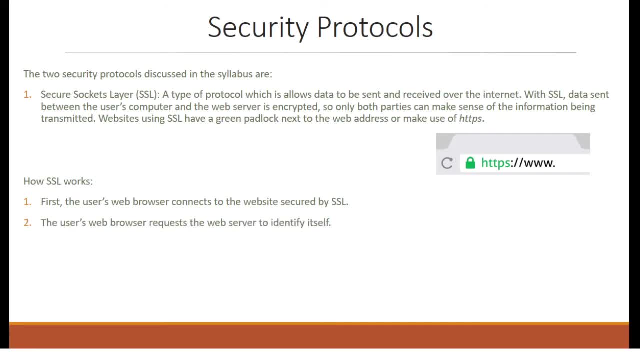 secured by ssl. the user's web browser requests the web server to identify itself. the web server sends a copy of its ssl certificate to the user's web browser. the web browser authenticates the certificate and sends a message to the web server to begin the communication process. the web server acknowledges this message. 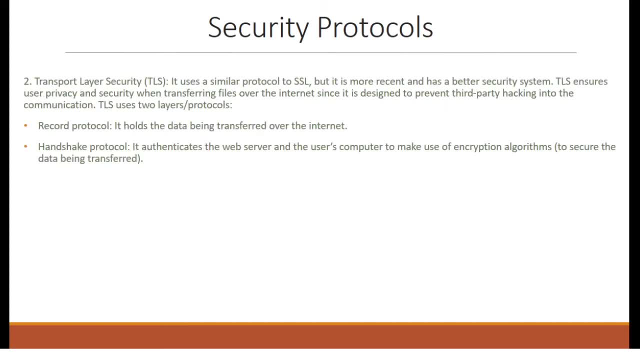 and the ssl encrypted two-way data transfer begins. the second security protocol is transport layer security, or tls. the third security protocol is the ssl protocol to ssl, but it is more recent and has a better security system. tls ensures user privacy and security when transferring files over the internet. 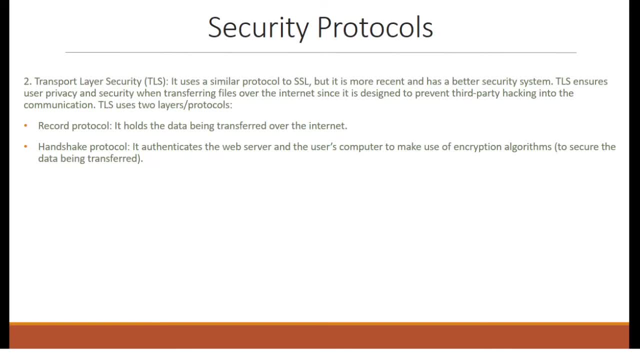 since it is designed to prevent third-party hacking into the communication. tls uses two layers or protocols. first, the record protocol. this holds the data being transferred over the internet to handshake protocol. the third security protocol is the ssl protocol, which is used to authenticate the web server and the user's computer to make use of encryption algorithms. 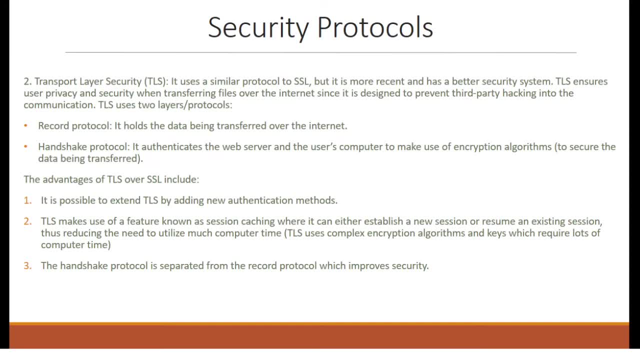 the advantages of tls over ssl include: it is possible to extend tls by adding new authentication methods. tls makes use of a feature known as session caching, where it can either establish a new session or resume an existing session, thus reducing the need to utilize much computer time. the handshake protocol is separated from the record protocol, which improves security. 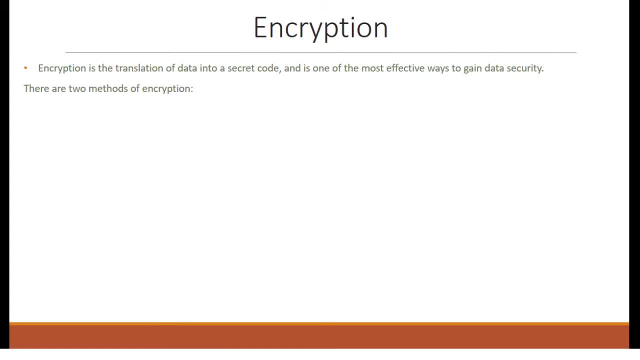 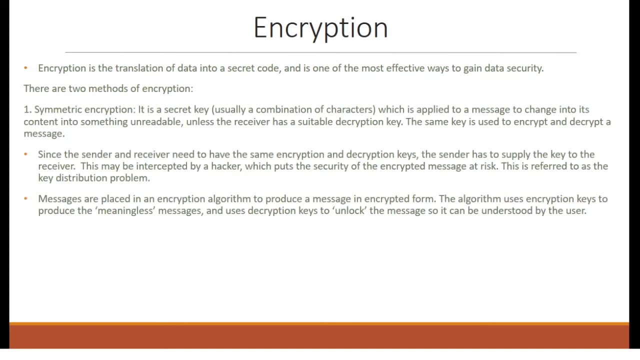 encryption. it is a translation of data into secret code and is one of the most effective ways to gain data security. there are actually two methods of encryption. it may seem confusing at first, so you can try to reread this part if you want to. first, symmetric encryption: it is a secret key, usually a combination of characters, which is 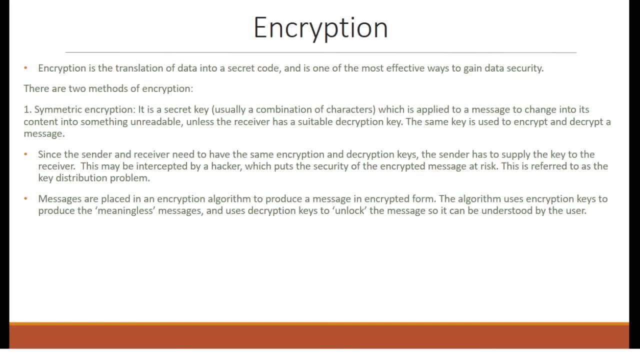 applied to a message to change its content into something unreadable, unless the receiver has a suitable decryption key. the same key is used to encrypt and decrypt a message, so only one key is used in this method of encryption, since the sender and receiver need to have the same encryption and decryption keys. since there's 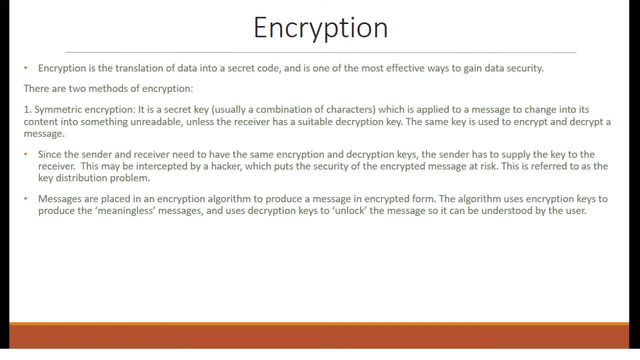 no key, the sender has to supply the key to the receiver. this may be intercepted by a hacker, which puts the security of the encrypted message at risk. this is referred to as a key distribution problem. messages are placed in an encryption algorithm to produce a message in encrypted form. 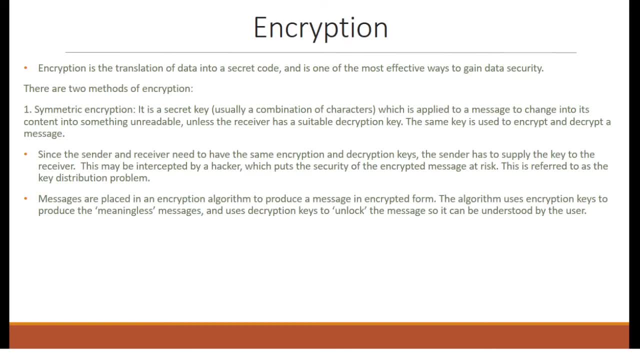 the algorithm uses encryption keys to produce the meaningless messages and uses decryption keys to unlock the message so it can be understood by the user. the decryption key is used to unlock the message so it can be understood by the user. to asymmetric encryption, it is also known as public key encryption and it is a more secure 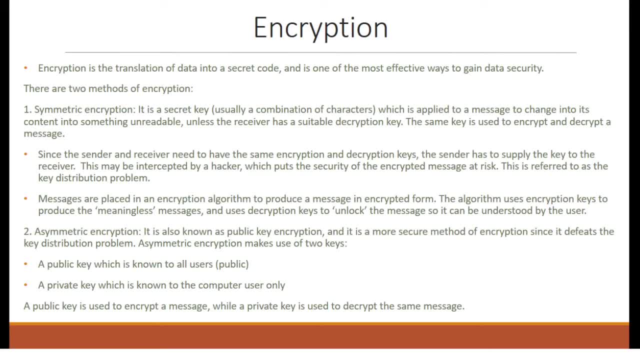 method of encryption, since it defeats the key distribution problem. asymmetric encryption makes use of two keys: a public key, which is known to all users, and a private key, which is known to the computer user. only a public key is used to encrypt a message, while a private key is. 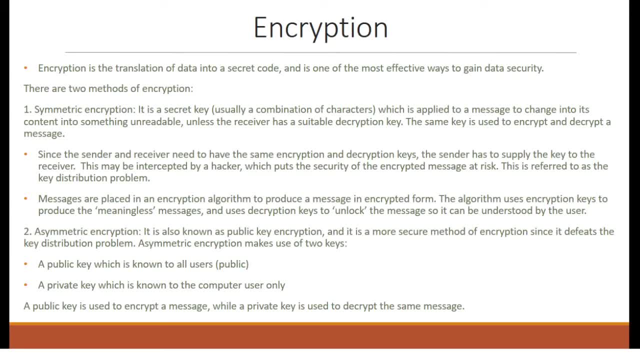 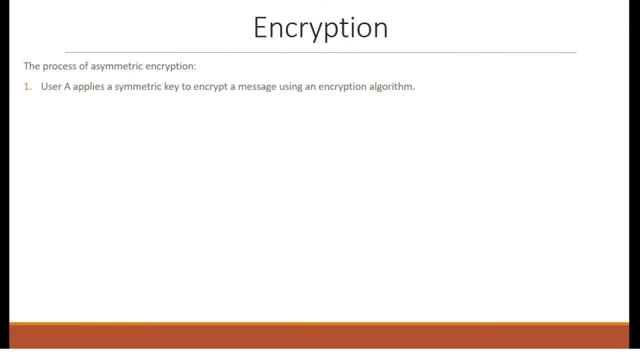 used to decrypt the same message: the process of asymmetric encryption. user a applies a symmetric key to encrypt a message using an encryption algorithm. the symmetric key is encrypted using the public key known to users a and b. user a transmits the message and symmetric key over the internet. user b decrypts the symmetric key using their own private key, the decrypted. 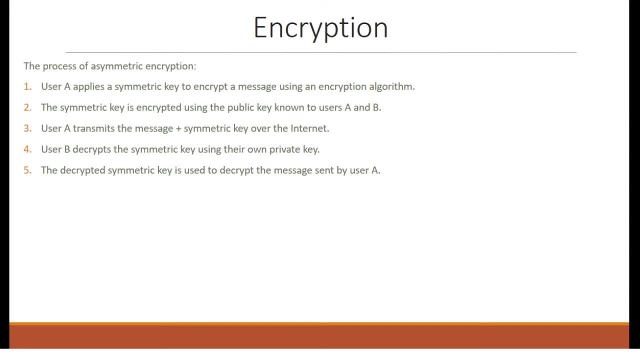 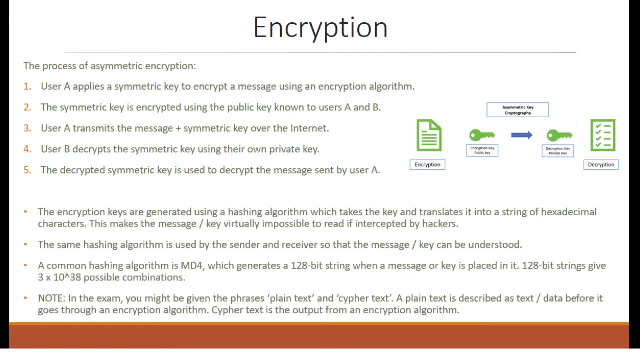 key is then used to decrypt the message sent by user a. the encryption keys are generated using a hashing algorithm which takes a key and translates it into a string of hexadecimal characters. this makes the message or key virtually impossible to read if intercepted by hackers. the same hashing 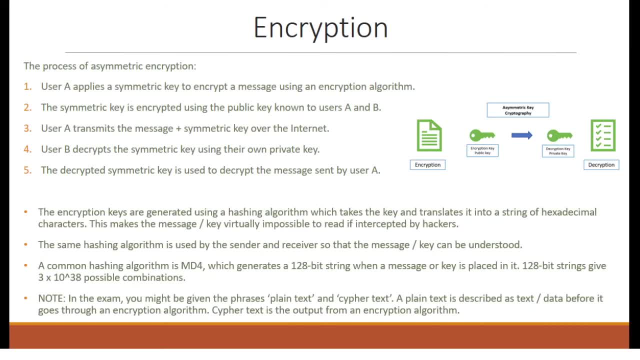 algorithm is used by the sender and receiver so that the message or key can be understood. a common hashing algorithm is md4, which generates a 128-bit string when a message or key is placed in it. 128-bit strings give 3 times 10 to the power, 38 possible combinations. 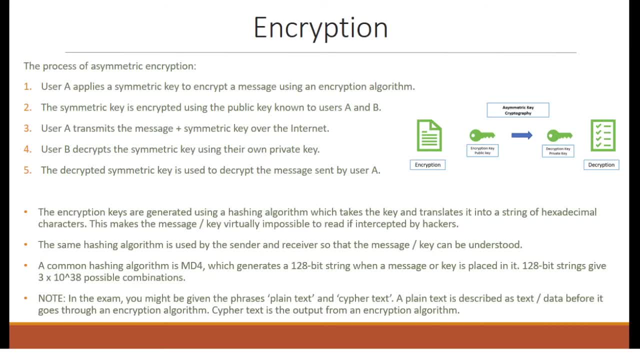 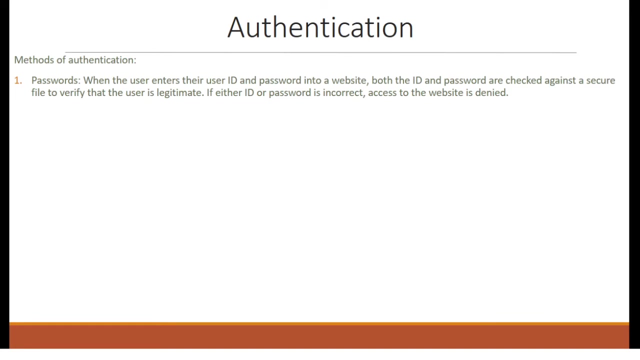 note in the exam you might be given the phrases plain text and ciphertext. a plain text is described as text or data before it goes to an encryption algorithm. ciphertext is the output from an encryption algorithm. moving on to the methods of authentication, authentication is basically the process of 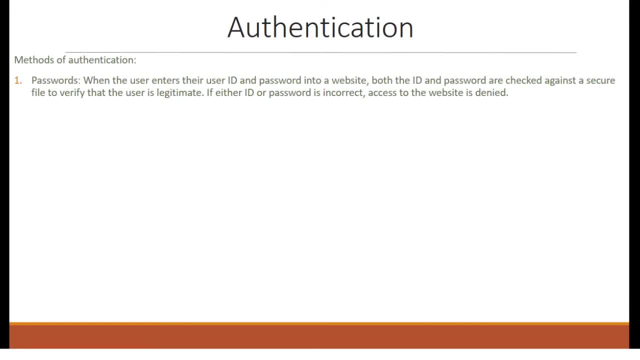 verifying the identity of a personal device. method 1- passwords. when the user enters their user id and password into a website, both the id and password are checked against a secure file to verify that the users legitimate. is either id or password is incorrect, access to the website is denied. 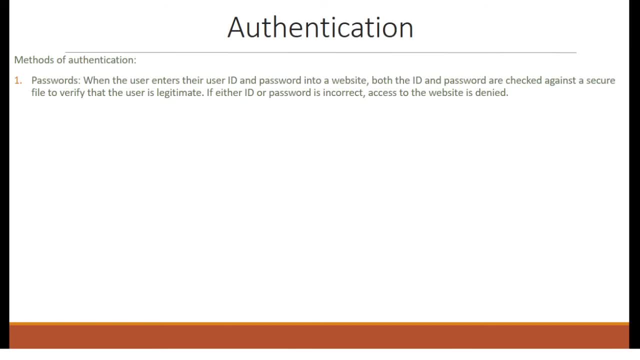 biometrics: it relies on the unique characteristics of human beings. examples include fingerprint scans, where images of fingerprint are compared against a list of scanned fingerprints stored in a database. if the fingerprint of the user matches, then access is granted. retina scans: it scans the pattern of blood vessels and blood. Sic ridicules measures solo出來 of blood vessels in the blood cell and administrator records the pattern of blood vessels and determines the risk of satin in the case ofому. 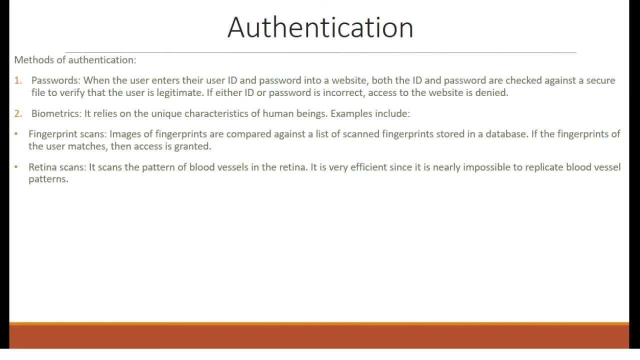 retina scans. it scans the pattern of blood vessels in the patienteloid- 체 beadsуй出来 vessels in the retina. It is very efficient, since it is nearly impossible to replicate blood vessel patterns. Digital Signatures: A method used to ensure that an electronic 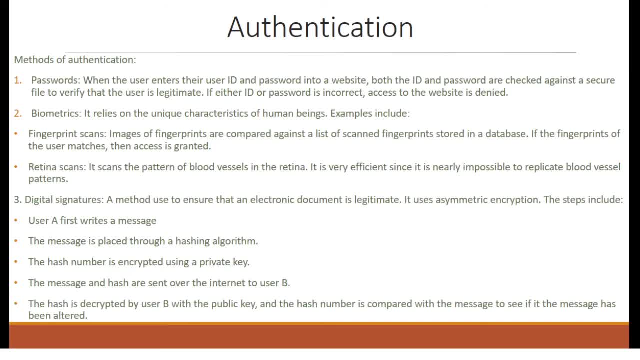 document is legitimate. It uses asymmetric encryption. The steps include: User A first writes a message. The message is placed through a hashing algorithm. The hash number is encrypted using a private key. The message and hash are sent over the Internet to User B. The hash is then decrypted by User B with the public key and the hash. 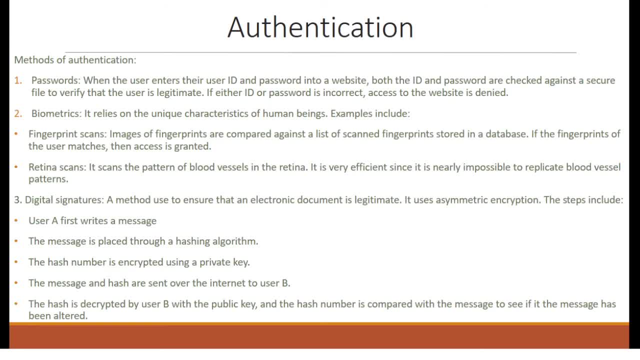 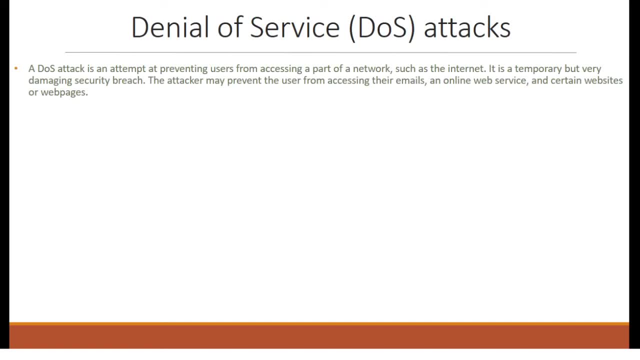 number is compared with the message to see if the message has been altered. Denial of Service Attack. A DOS attack is an attempt at preventing users from accessing a part of a network, such as the Internet. It is a technique to avoid a network that is not connected with a network. This is: 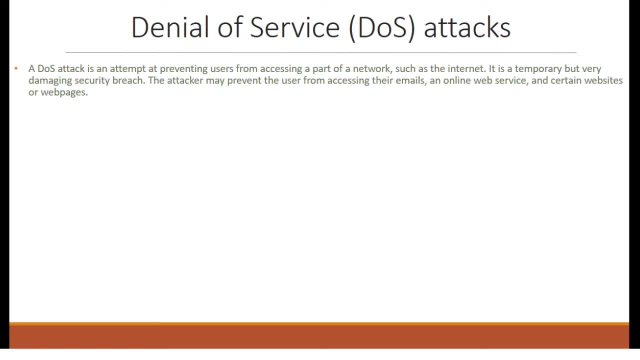 temporary but very damaging security breach. The attacker may prevent the user from accessing their emails, an online web service and certain websites or web pages. A DOS attack is performed by flooding a website or web page with useless traffic. A web server can only handle a finite amount of requests, so 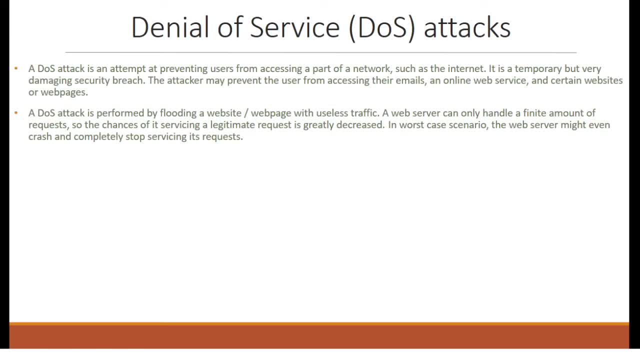 the chances of it servicing a legitimate request is greatly decreased. In the worst case scenario, the web server may even crash and completely stop servicing its requests. A DOS attack can also happen to user's email by sending tons of spam emails to user's email account, Since ISPs only allow a specific 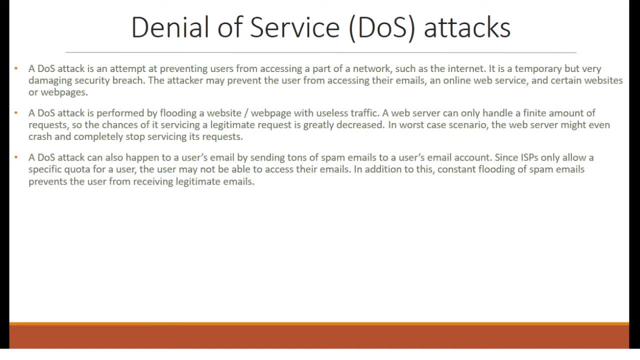 quota to a user, the user may not be able to access their emails. In addition to this, constant flooding of spam emails prevents the users from receiving receiving legitimate emails. Users can prevent these attacks to a certain degree by applying email filters to filter out spam emails, using a firewall to restrict traffic and using an updated virus checker. 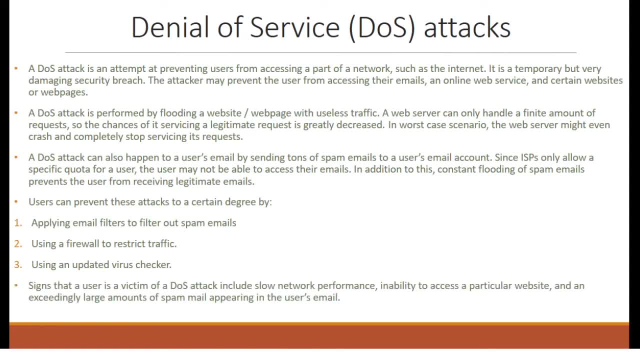 Signs that a user is a victim of a DOS attack include slow network performance, inability to access a particular website and an exceedingly large amount of spam email appearing in the user's email. Now let's discuss about the applications of the security features previously mentioned. 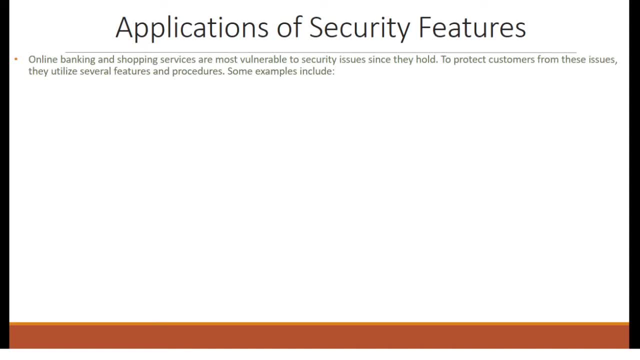 Online banking and shopping services are most vulnerable to security issues, since they hold sensitive data. To protect customers from these issues, they utilize several features and procedures. Banking services use SSL encryption to protect the customer's personal details. Many banks use a 10-12 digit code which is unique to each customer. 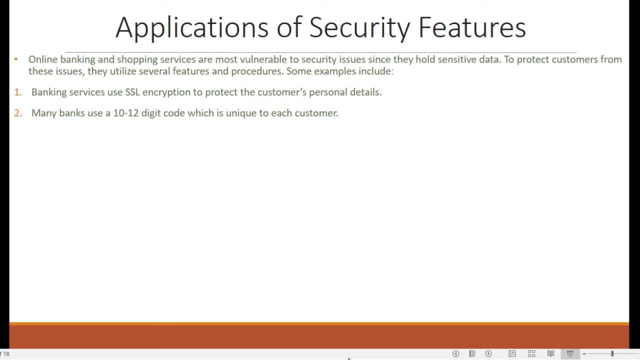 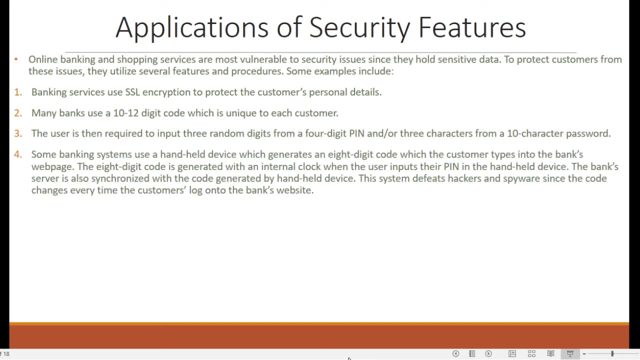 This code is entered when the user visits the website. The user is then required to input 3 random digits from a 4-digit PIN and or 3 characters from a 10-character password. Some banking systems use a handheld device which generates an 8-digit code which the 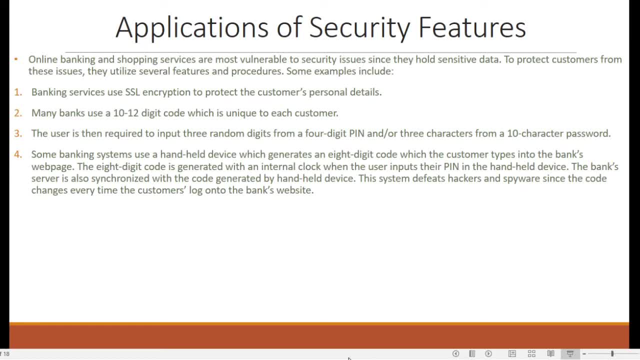 customer then types into the bank's website, The 8-digit code is generated with an internal clock. when the user inputs their PIN into the handheld device, The bank's server is also synchronized with the code generated by the handheld device. The system defeats hackers and spyware, since the code changes every time the customer allows. 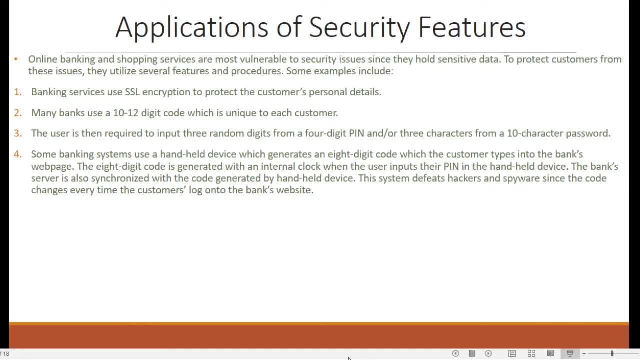 to log onto the bank's website, We can see an example of a handheld keypad. to the right, Customers are then asked to input certain characters from their password. using drop-down boxes, The user selects the required characters using a mouse. This defeats spyware and keyloggers, since it eliminates the use of a keyboard. 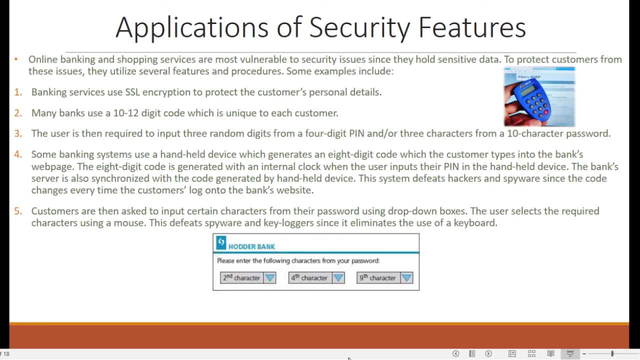 Sometimes the website asks the user to type the password into the keypad. The user then asks the bank to type the password into the keypad. The bank then asks the bank to type the password into the keypad. Did the user type in the password for a personal data, such as when was the last time you? 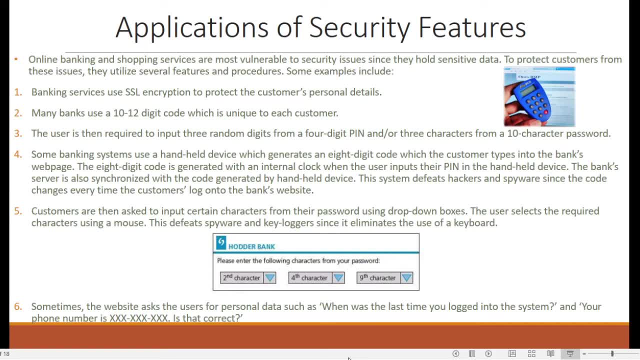 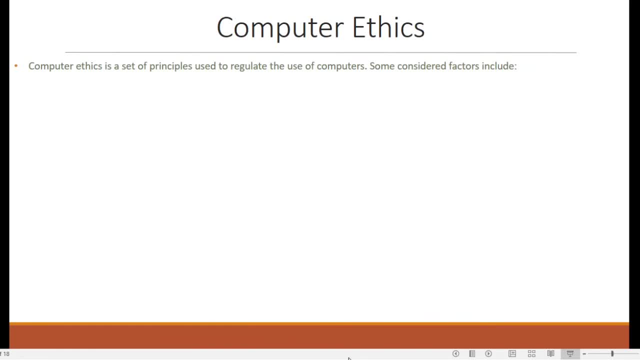 logged into the system and your phone number's xxx. Is that correct? Computer ethics is a set of principles used to regulate the use of computers. Some considered factors include intellectual property rights, the right to give people credit for their work, For example, copyright laws. 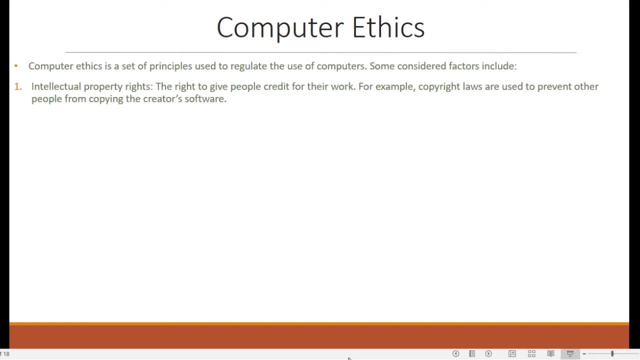 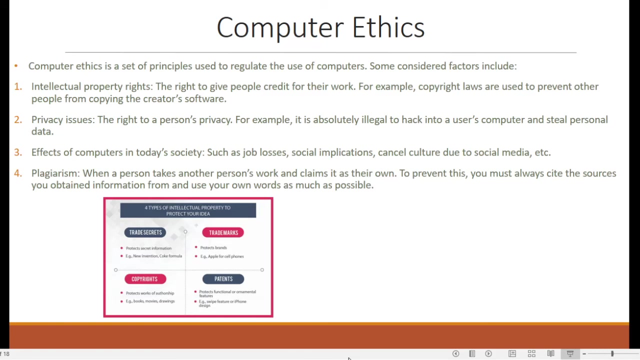 to prevent other people from copying the creator. software privacy issues the right to a person's privacy. for example, it is absolutely illegal to hack into a user's computer and steal personal data. effects on computers in today's society, such as job losses, social implications and cancel culture due to social media plagiarism when a user takes another person's work and claims it. 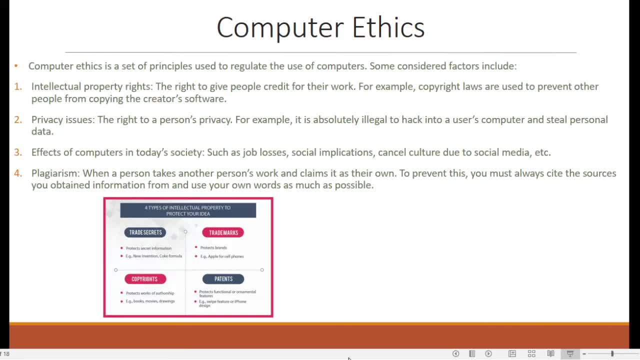 as their own. to prevent this, you must always cite the sources you obtain information from and use your own words as much as possible. the example on the right shows how you can use your own words, but i do not recommend writing slangs for your essays. finally, the types of software. 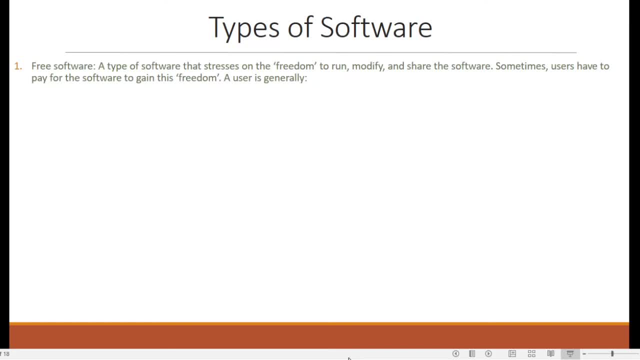 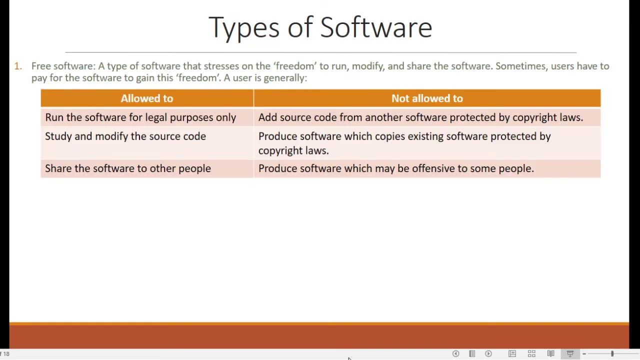 free software, a type of software that stresses on the freedom to run, modify and share the software. sometimes users have to pay for the software to gain this freedom. a user is generally allowed to run the software for legal purposes, study and modify the source code and share the software to. 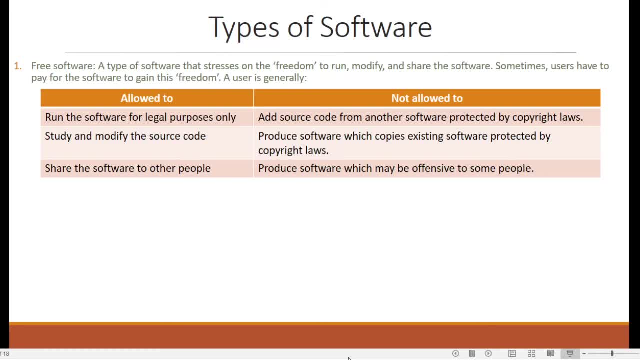 other people. however, the user is not allowed to add source code from another software protected by copyright laws, produce software which copies existing software protected by copyright laws and produce software which may be offensive to some people. freeware: a type of software which can be downloaded free of charge. 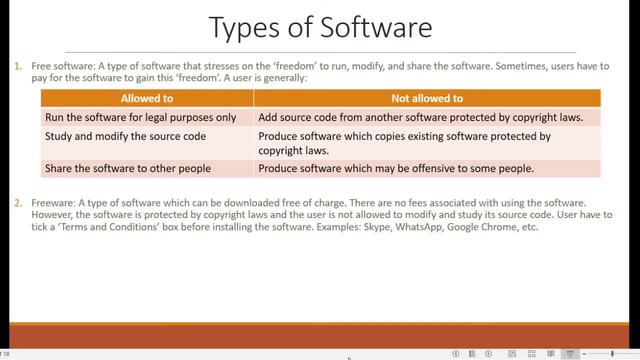 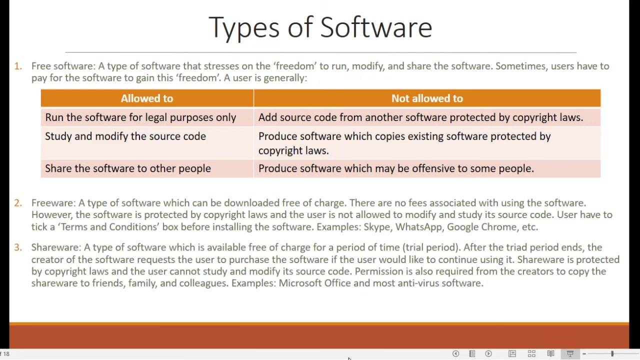 there are no fees associated with using the software. however, the software is protected by copyright laws and the user is not allowed to modify and study source code. users have to take a terms and conditions box before installing the software. examples include skype, whatsapp, google, chrome, etc. shareware, a type of software which is available. 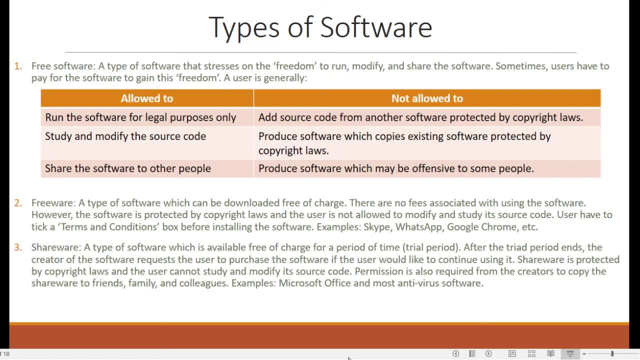 free of charge for a period of time. this is known as a trial period. after the trial period ends, the creator of the software requests the user to purchase the software if they if the user would like to continue using it. here's a basic overview of how to use freeware.